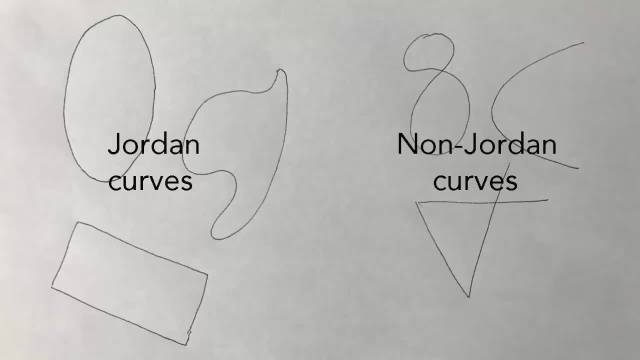 Here's another outstanding mystery, understandable with just pen and paper for you to while away the hours. Draw a closed loop. It can be any shape you like, just so long as it's a simple loop, which means that it doesn't cross over itself and it has no loose ends. 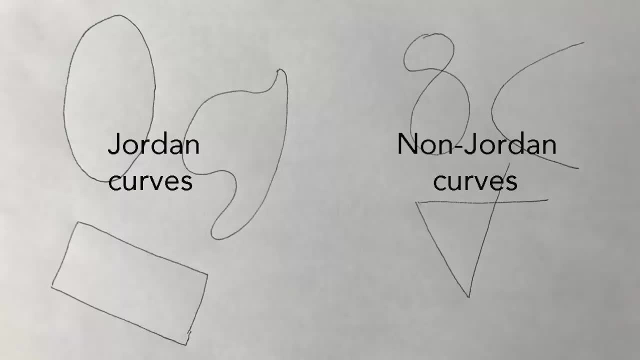 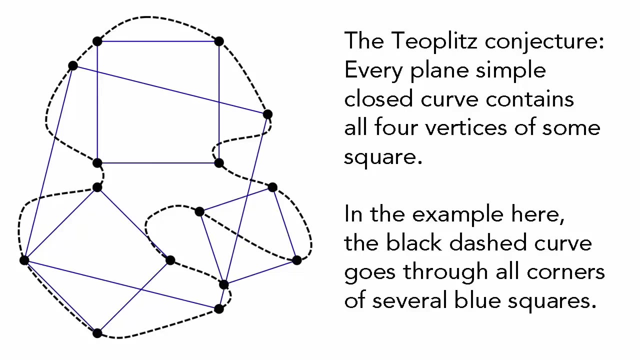 We call such a loop a Jordan Curve. In 1911, the German mathematician Otto Toplitz put forward this proposal. Every Jordan Curve contains an inscribed square, Known as the Toplitz conjecture or inscribed square hypothesis. the suggestion is that inside any simple loop you can always draw a square. 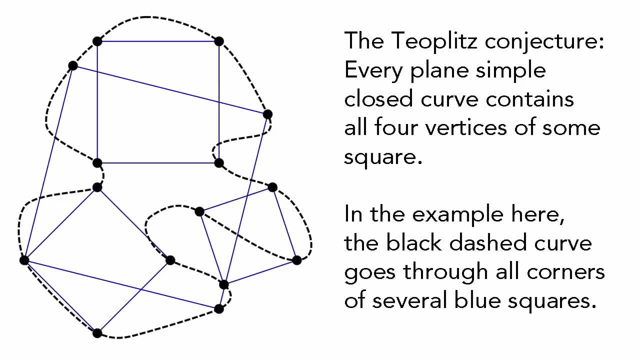 so that all four corners touch the loop. It's easy to draw examples where this is true, a perfect circle being the most obvious case. but the question is: does the Toplitz conjecture hold for every possible Jordan Curve? You can amuse yourself all day long drawing different loops. 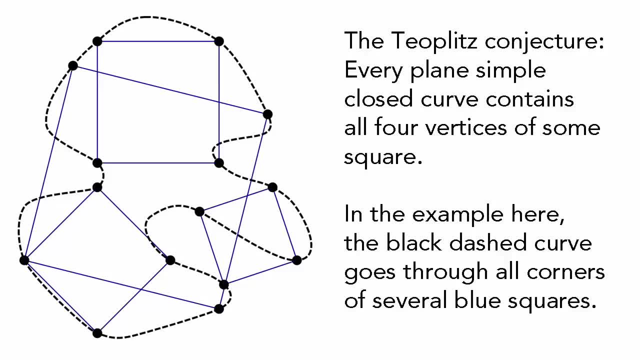 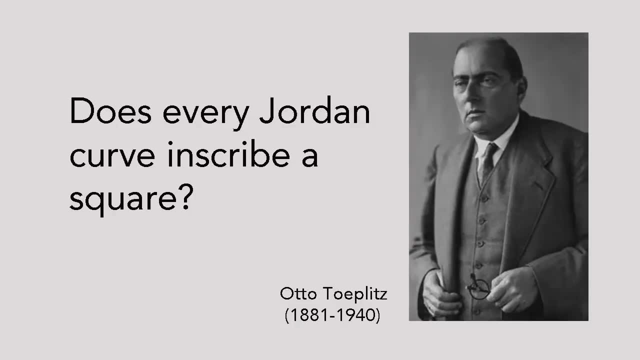 and trying to find places where a square will exactly fit, but that proves nothing. What about the infinitely many other Jordan Curves that you haven't had? Have you ever had time to draw or test? The Toplitz conjecture has been shown to hold for a large class of Jordan Curves. 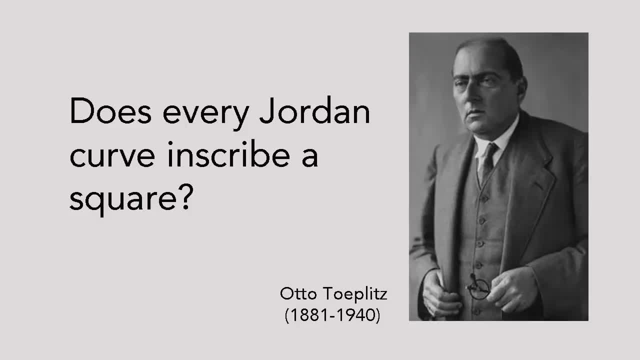 namely those that are convex and smooth. The key point about a convex curve is that a straight line drawn between any two points on the curve will never cross over it. Smooth in the mathematical sense means that the slope of a line that just touches the curve, a tangent 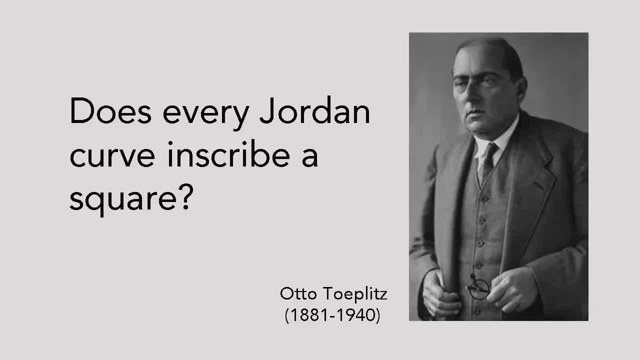 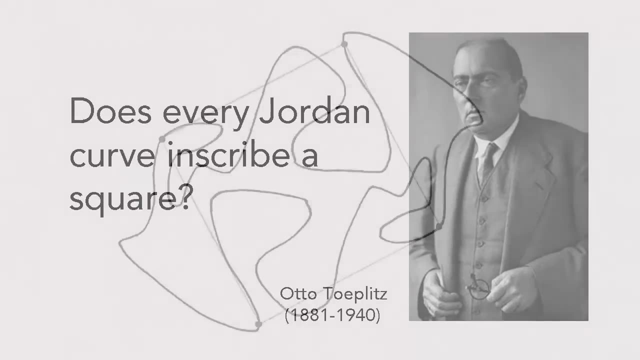 never jumps abruptly from one point to the next. In plain language, the curve has no corners, But Jordan, Curves can be both concave and non-smooth, and this complicates the problem immensely. In fact, mathematicians have shown that the equivalent of the Toplitz conjecture 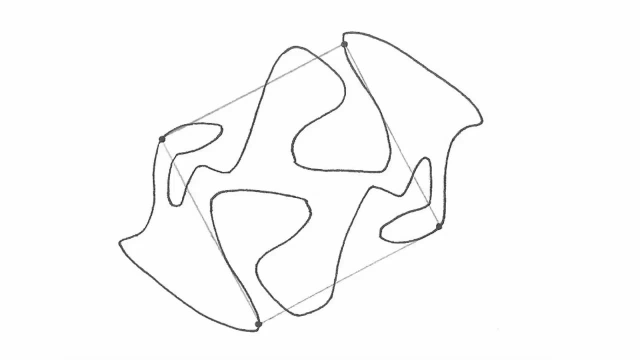 holds true for every type of Jordan Curve in the case of a number of other shapes, including triangles and rectangles, But squares, it turns out, are trickier, And so the hunt is still on for a proof that works for every possible curve. 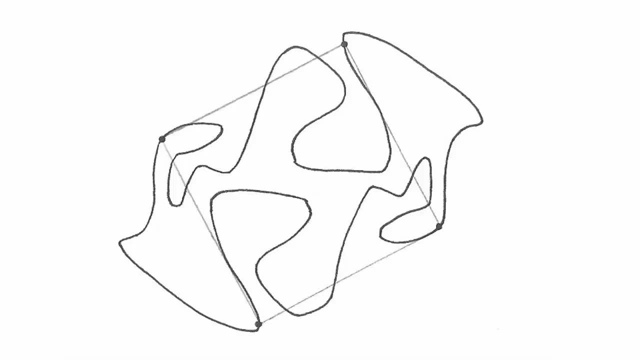 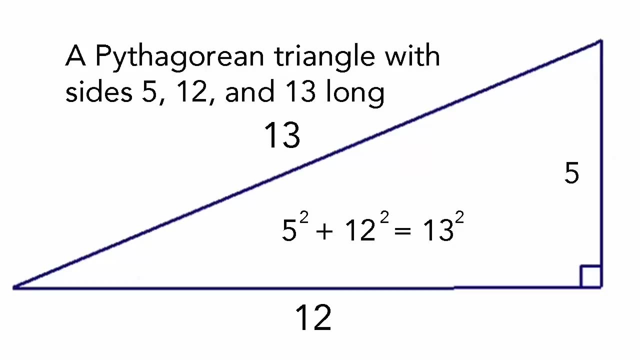 even those that have pointy bits or bow outwards. Stepping up a dimension brings us to an unsolved problem. that takes us back to our school days. At some point we all learn about Pythagoras' theorem in a right-angled triangle. 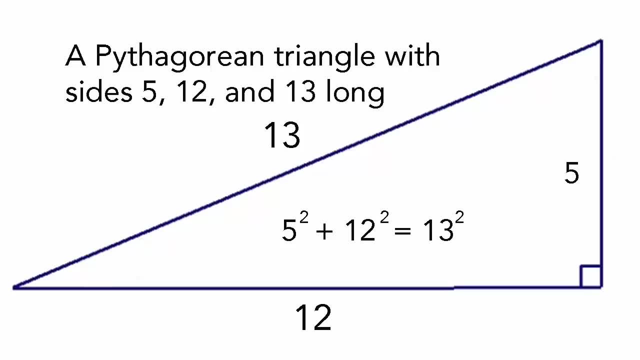 the square of the hypotenuse, the longest side equals the sum of the squares of the other two sides. A Pythagorean triangle is a special case where all the sides have a whole number of lengths. Familiar examples are the 3-4-5 triangle. 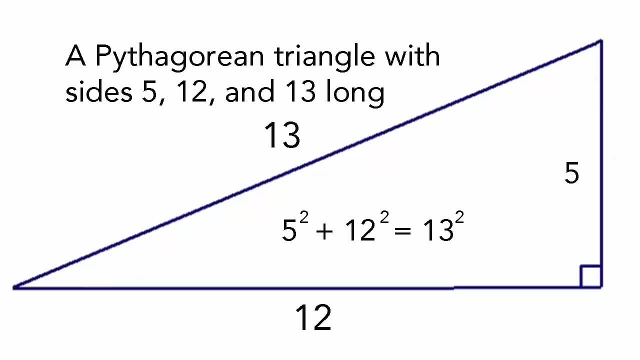 because 3 squared plus 4 squared equals 5 squared and the 5-12-13 triangle In three dimensions. Pythagoras' theorem works equally well, but we need four numbers to take account of the lengths in the X, Y and Z directions. 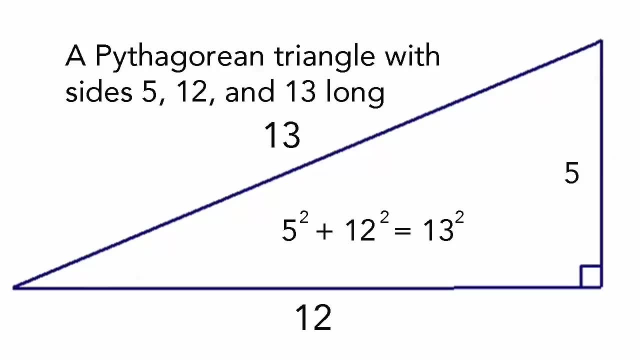 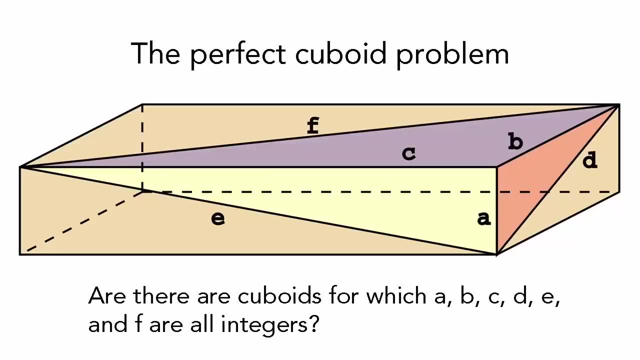 plus that of the diagonal connecting the endpoints. This brings us to the so-called perfect cuboid problem. Just as there are Pythagorean triangles where the lengths of all three sides are whole numbers, so there are some cuboids where the three edges in the X, Y and Z directions 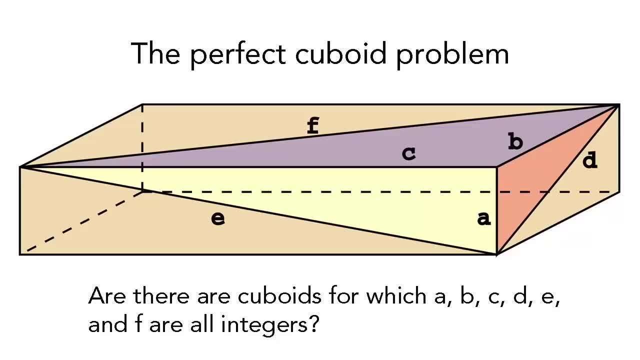 and the spatial diagonal across the box. four lengths in all have integer values, But each of the three faces of a cuboid also has a diagonal. The perfect cuboid problem asks: are there any boxes where all seven of these numbers, giving the lengths of the three edges? 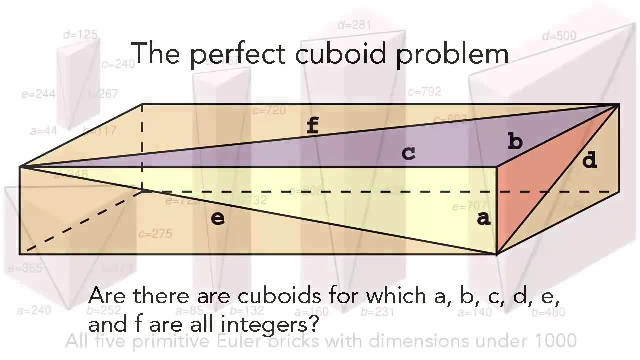 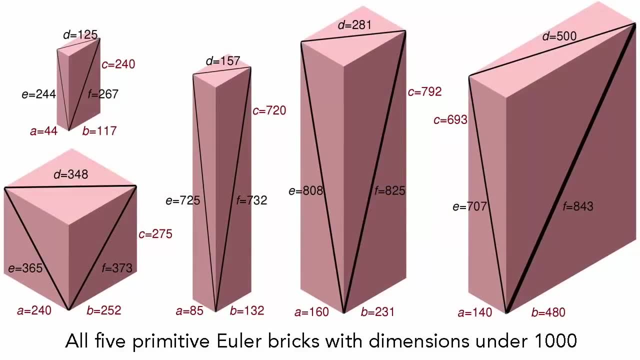 plus, the four diagonals are whole numbers. Mathematicians have come up with a few near-misses. The shape known as an Euler brick is like a perfect cuboid, but its spatial diagonal doesn't have to be an integer length. The easing of this restriction allows solutions to be found. 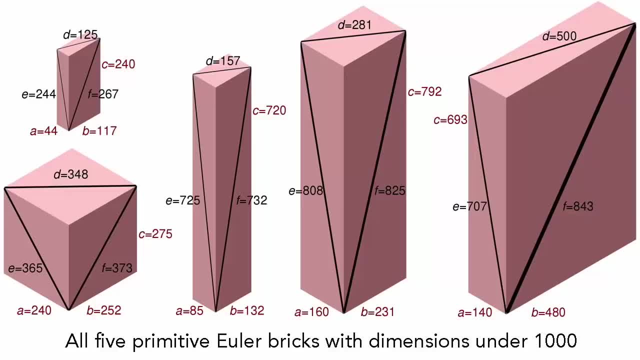 The smallest Euler brick was discovered not by Euler himself but by a contemporary of his, the German mathematician Paul Halcke, in 1719.. It has edges of length 44,, 117 and 240, and face diagonals of length 125, 244 and 267.